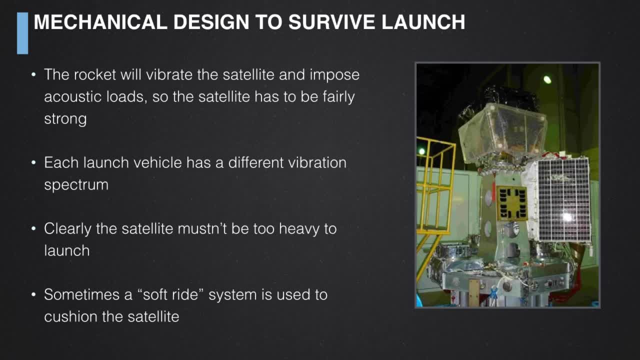 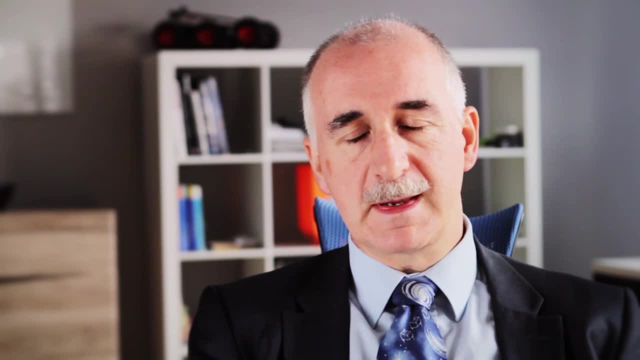 It's quite loud in the fairing of a launch vehicle. So potentially you have to design your spacecraft to withstand those loads And each different launch phase is going to be different. So you're going to have to design your spacecraft to withstand those loads And each different launch phase is going to have to withstand those loads. 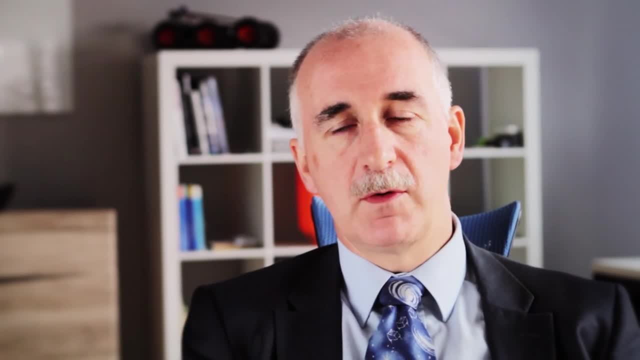 And each different launch phase is going to have to withstand those loads. You'll have to create a structure for the launch So the launch vehicle has a different vibration spectrum And you can, if you know the vibration spectrum, design a structure that doesn't. 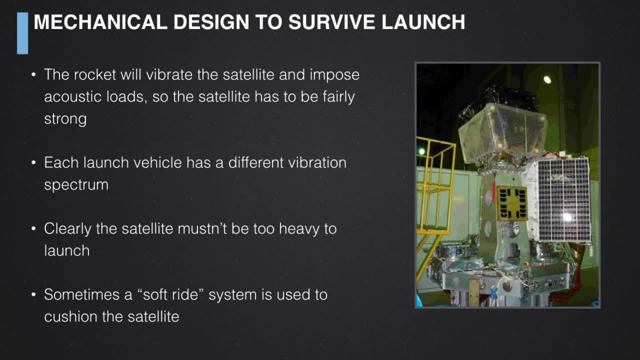 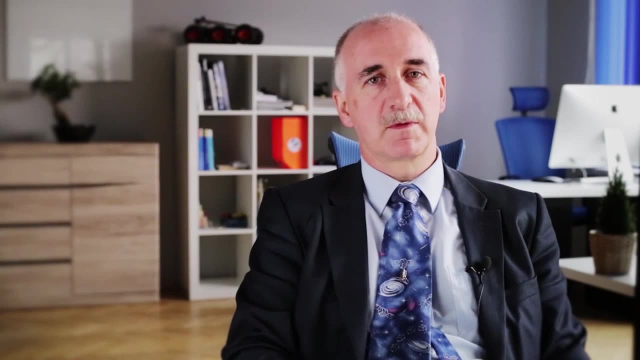 resonate at the particular frequency of the launch vehicle that you're planning to use. One of the issues that satellite technology has faced over the years is because we're launching relatively small spacecraft. we tend to be hitchhiker payloads- secondary payloads- on many launch vehicles. 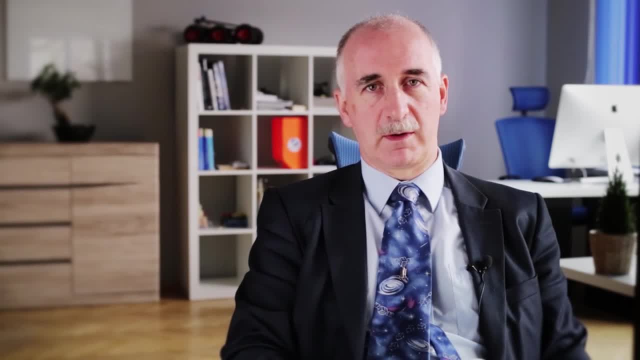 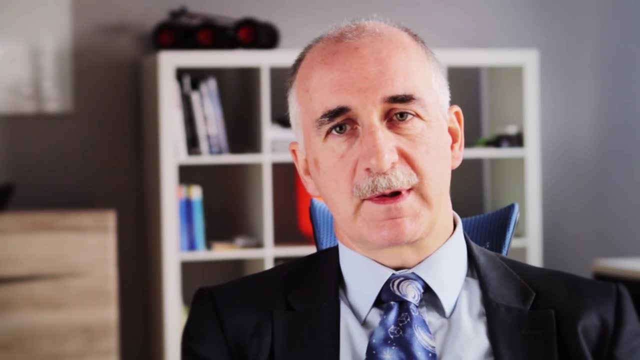 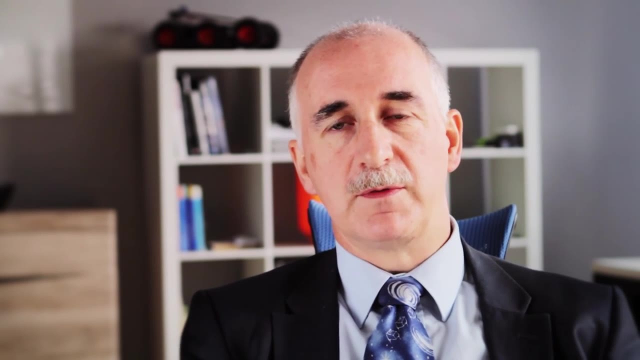 And, as a result, we don't start- start out when we are originally designing the mission, with a knowledge of which vehicle we'll definitely be flying on. So what this has led us to do is to design spacecraft structures that are able to cope with the vibration loads imposed by a variety of different launch vehicles. 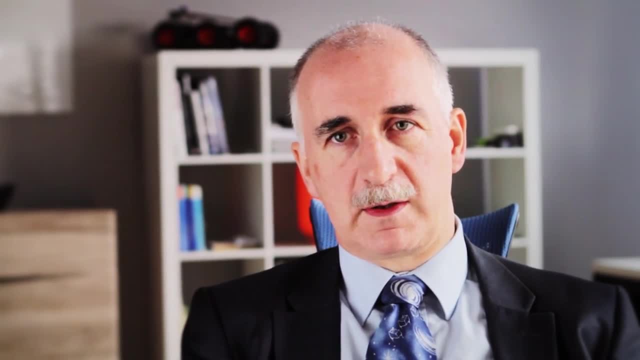 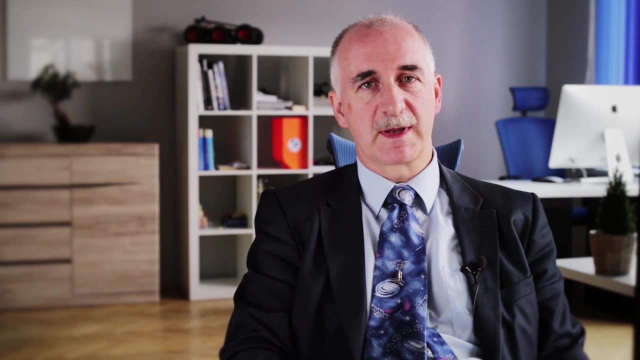 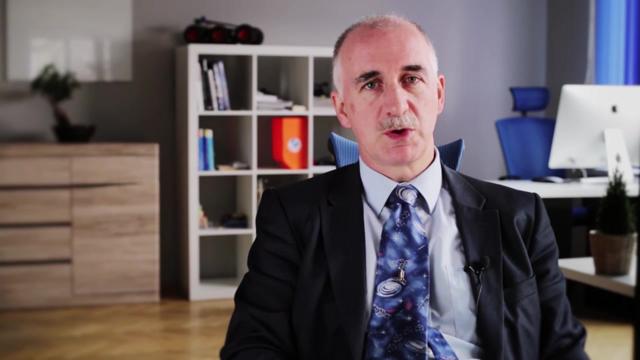 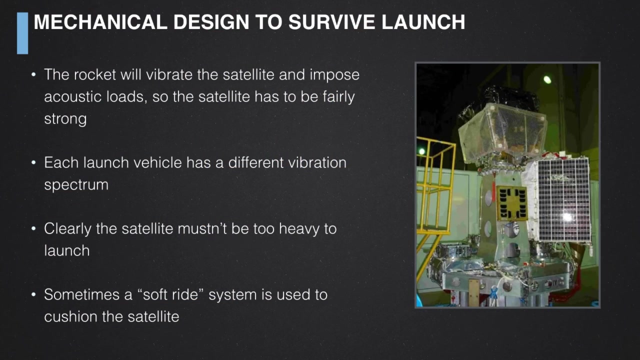 As you might imagine, that leads to a design that is perhaps over-designed for any given launch vehicle, but is nevertheless able to withstand the vibration effects of many different vehicles, which means that we can choose which launch vehicle we eventually go into orbit on. There are occasions where the payload of the mission actually demands that we do even more. 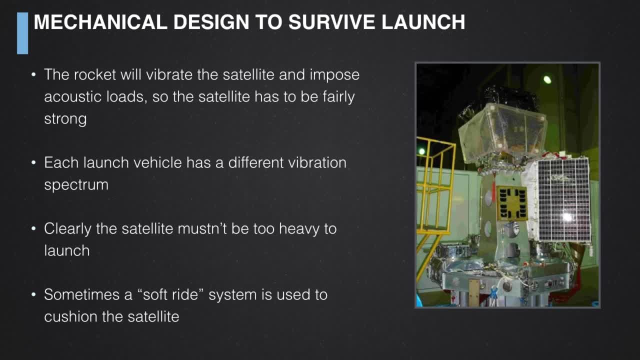 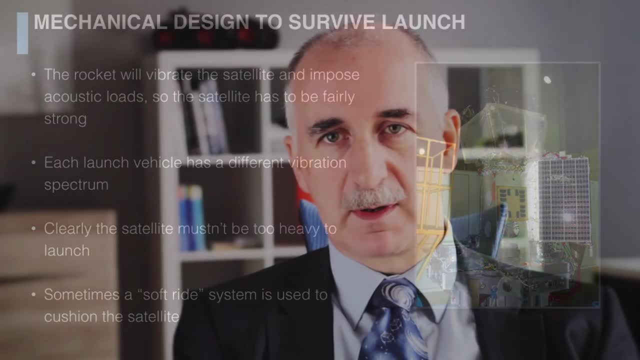 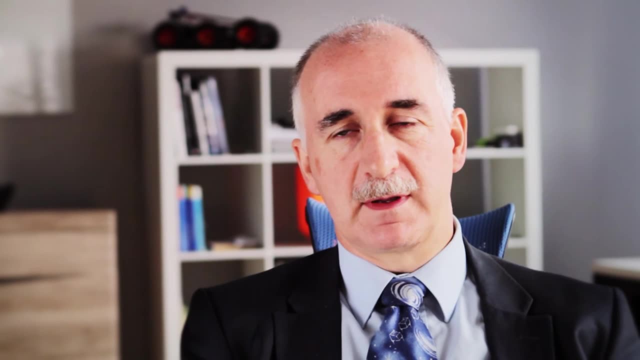 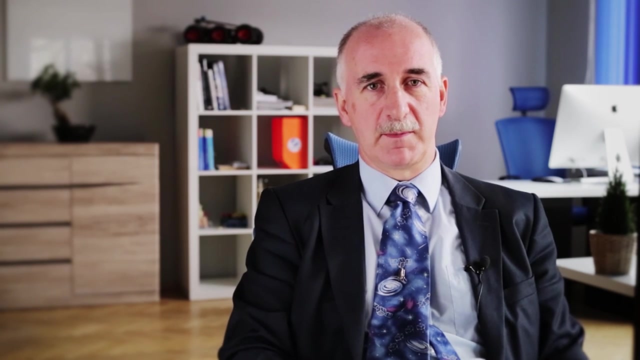 in terms of mechanical design. The satellite illustrated on this slide is a mission called Topsat. It had a very sophisticated three mirror astigmatic camera. An important feature of that is that three mirror astigmatic designs are quite hard to align, so the spacecraft had to essentially 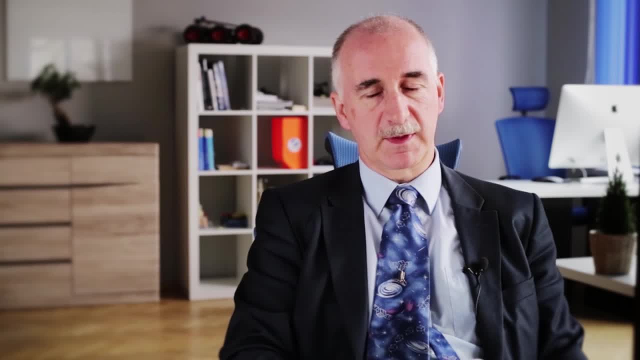 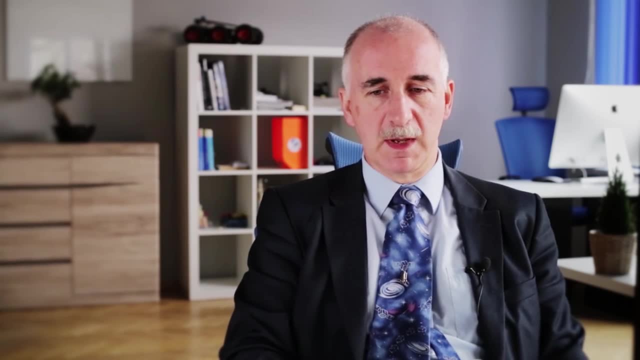 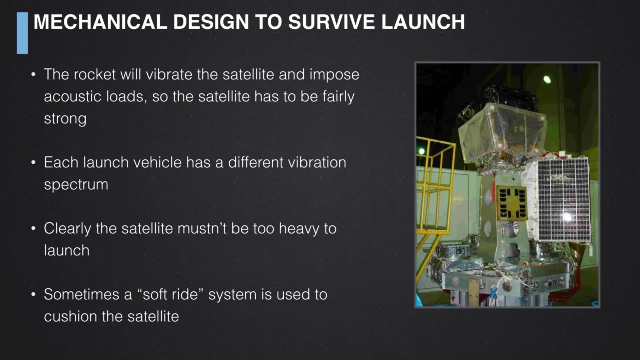 have its focus locked down before launch, and the last thing we wanted was for the launch vehicle to shake the mirrors out of alignment during the launch phase. So what we did in this case was inserted an interface between the launch vehicle and the satellite itself, which is called a soft ride system. The technical definition of it is a soft ride system When 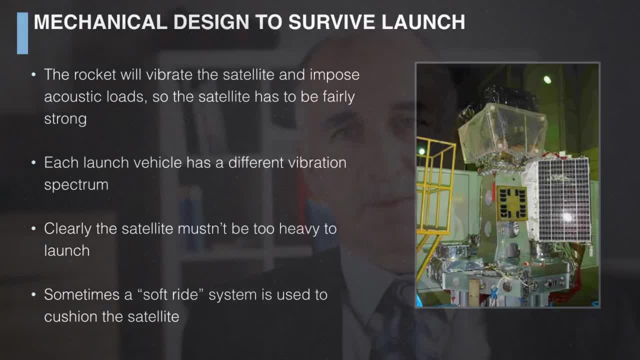 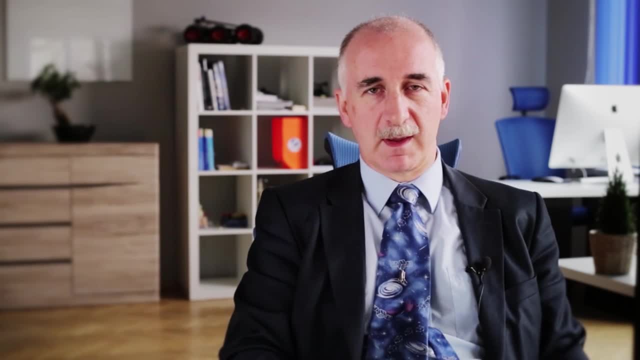 it was described to me first. it, which called a, called a set of magic rubber washers. The magic is choosing the right rubber materials so that it damps out the vibrations around a surface of the launch vehicle, rather than turning the whole system into a trampoline and making 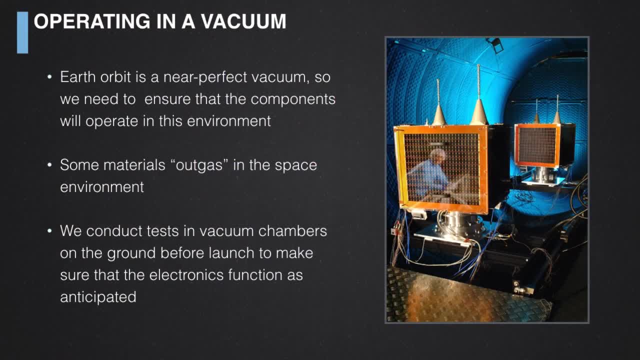 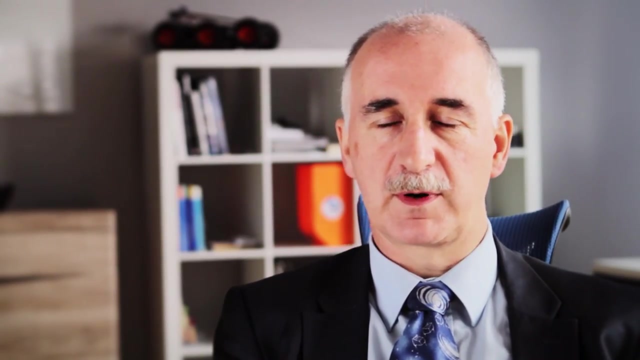 the vibration situation much worse. The satellite will arrive in space and then obviously you need to be able to convince yourself that the satellite will operate successfully in a vacuum. We take an awful lot of components from the terrestrial microelectronics world and they're, in general, not designed to operate in vacuums. they're designed to operate in mobile phones. 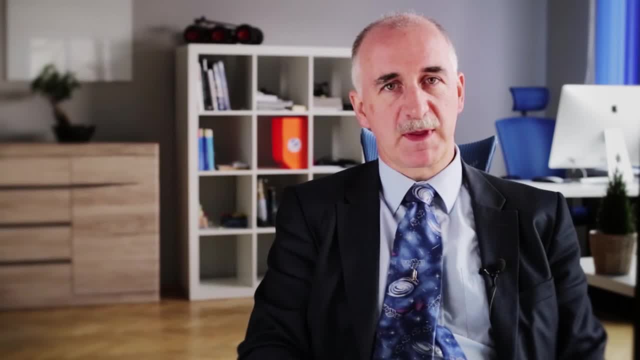 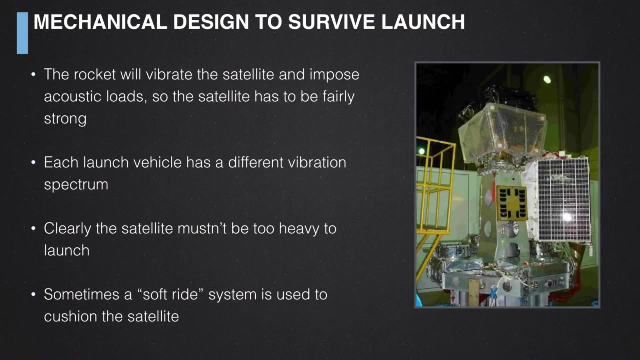 and laptop computers, etc. And some of the packaging of those devices is inappropriate for the space environment. The materials outgas when they get into a vacuum environment. It's important to make sure that anything that does outgas on your spacecraft doesn't end up coating your optics and making the system not function properly. 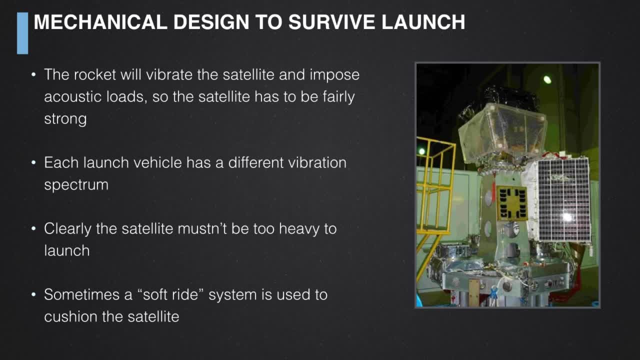 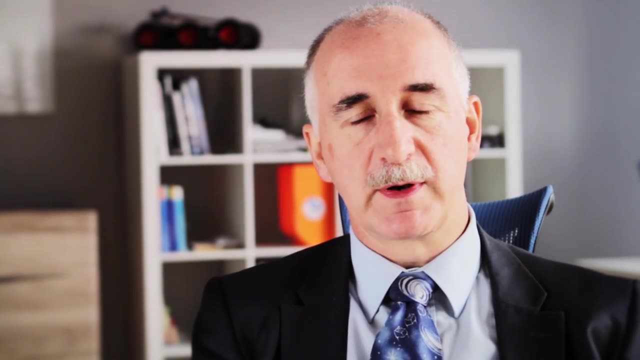 Thank you. And so we conduct tests in vacuum chambers on the ground to try and make sure that we're not using inappropriate materials before we launch. All satellites are going to need power, and most satellites these days, especially ones in orbit around the Earth, use solar panels. 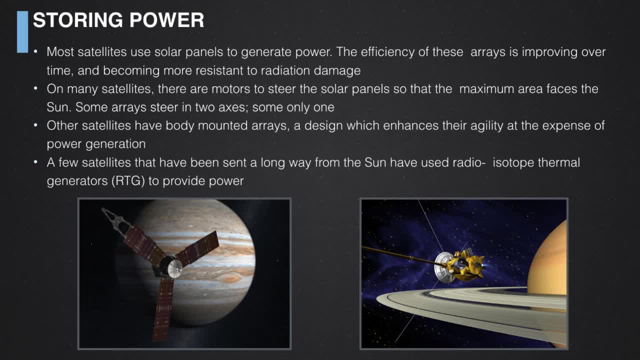 As we've moved from silicon-based semiconductors to gallium arsenide, the efficiencies of those solar cells has improved, With the result that we can do more with the satellite, because for a given array area we have more power. A lot of satellites have steerable solar arrays. 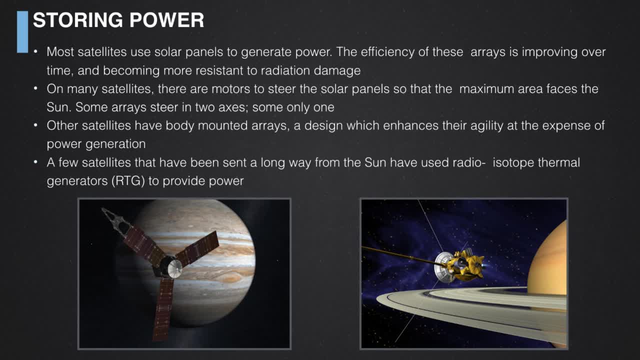 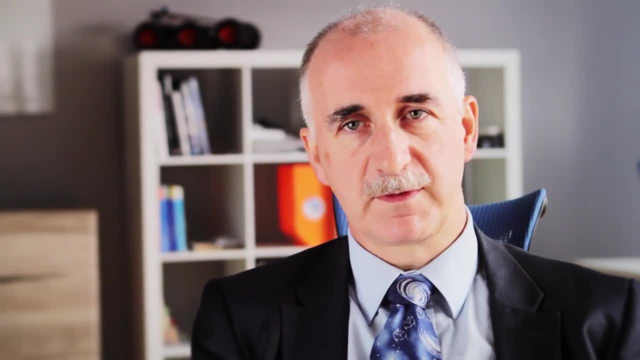 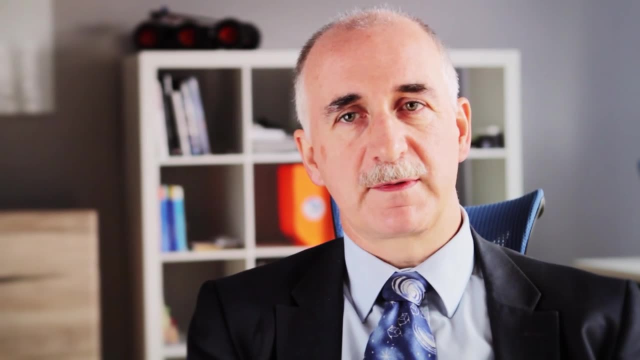 That isn't so often the case for the missions that we've built at Surrey. We've tended to use body-mounted solar panels, which allow the satellites to have considerably more agility than their bigger cousins. That obviously limits to some extent the amount of power you're able to generate on. 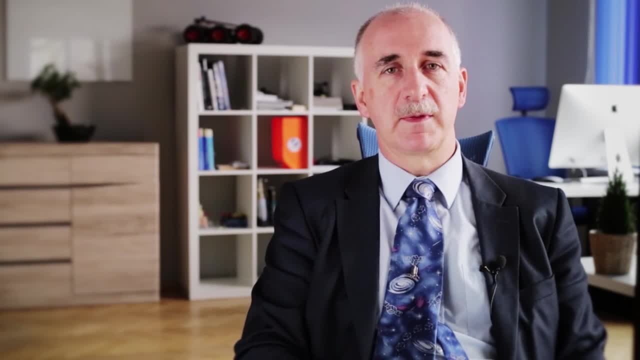 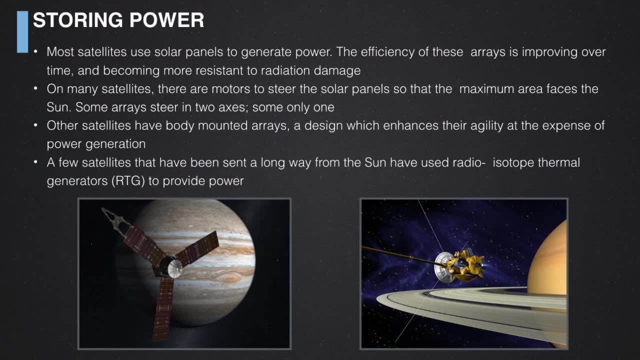 the spacecraft, but we've found that the trade-off works in our favour in many cases. The mission illustrated on the lower left of this slide is the NASA Juno mission, which is heading out to Jupiter at the moment. You'll notice that it has solar panels. 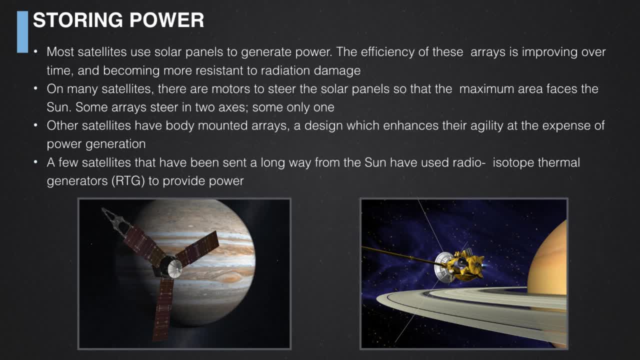 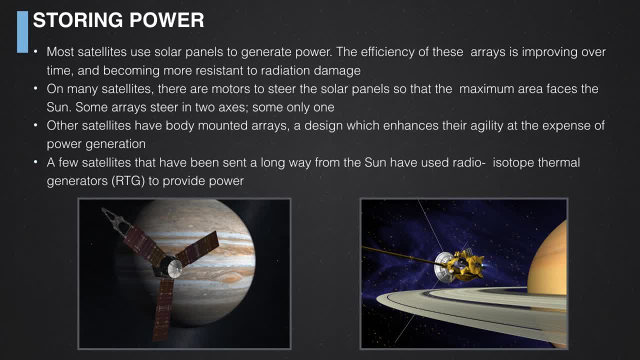 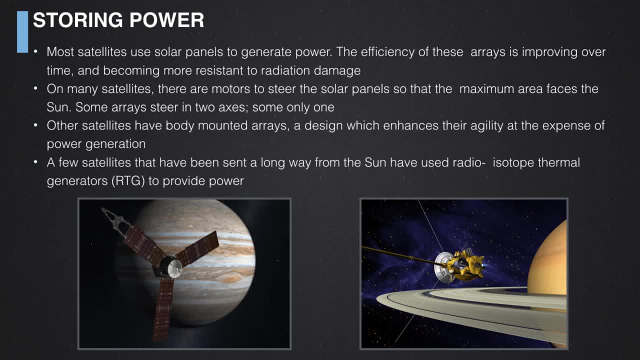 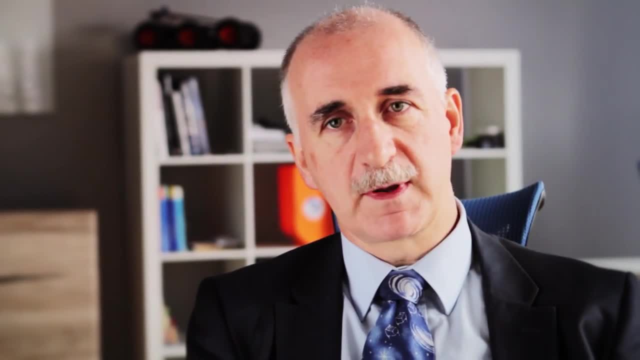 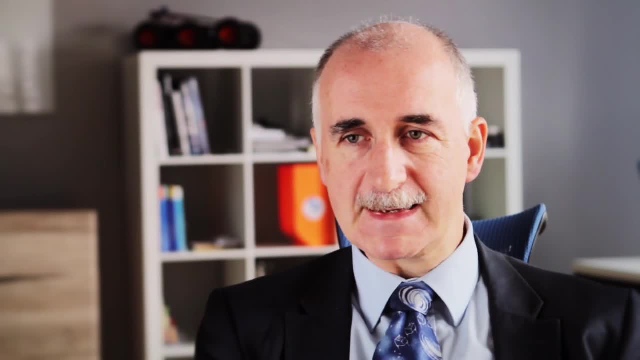 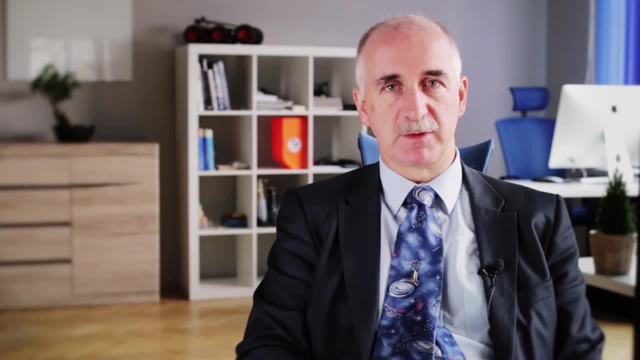 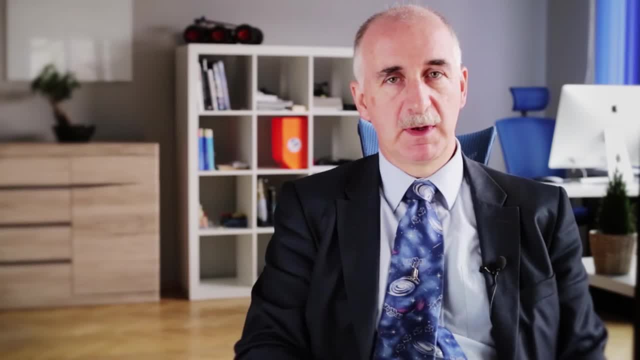 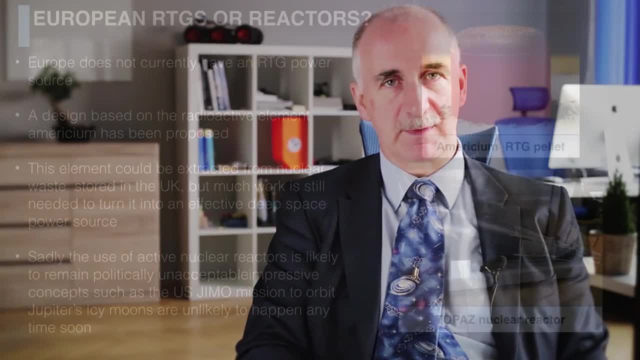 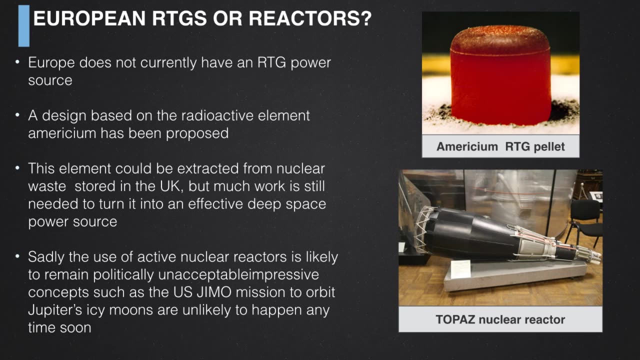 It's the first mission to go beyond Mars that has solar panels, generates heat and is used to power the spacecraft, So this is a concept that's being looked at in Europe at the moment. We don't have nuclear power in space in Europe at the moment, but although the American RTGs that have been used in the 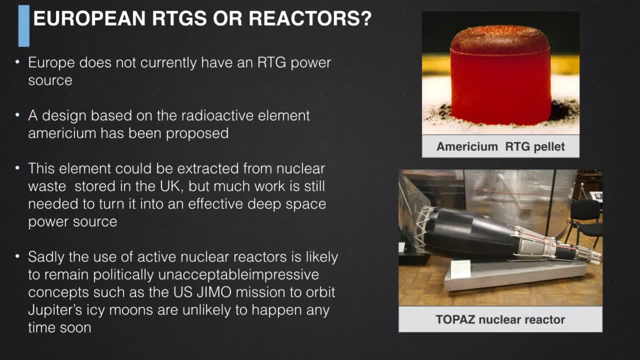 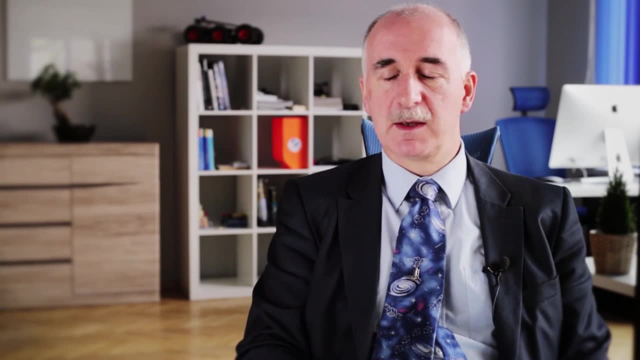 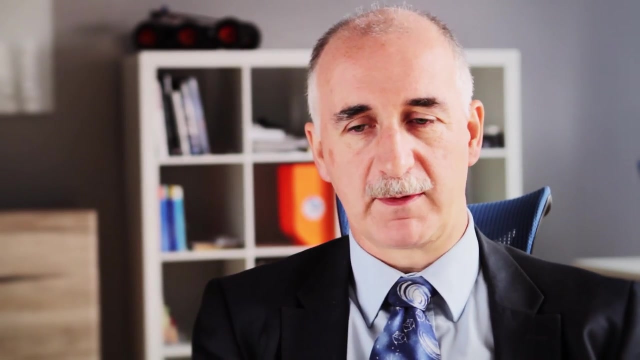 past have used plutonium as the radioactive element. Europe actually has a potential source in an element called an americium, which is in various waste stockpiles, some of which are held in the UK, which could be extracted and turned into fuel pellets that would similarly generate heat and therefore power. 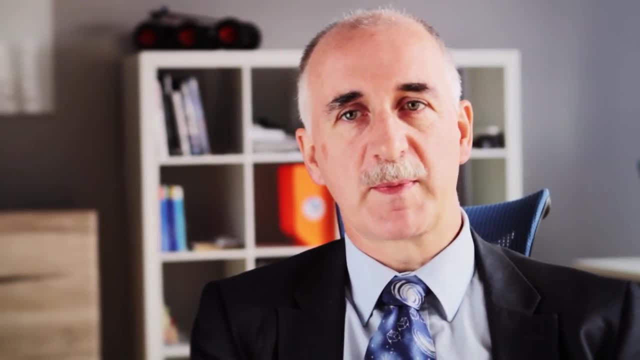 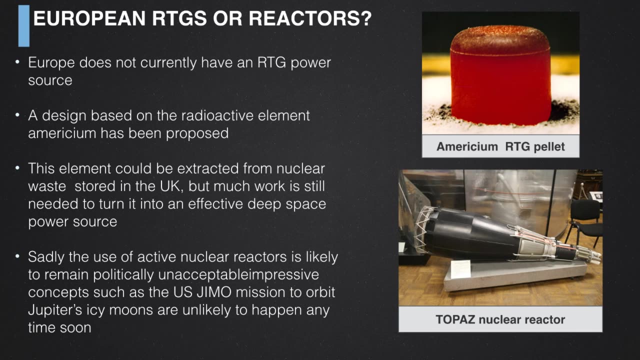 spacecraft, So we might be able to do deep space missions in Europe if we were able to develop this technology. and there are various steps that are required to make that technology work. The first thing to do would be to create the fuel pellets and then move on to creating suitable structures, heat exchanges, etc. to 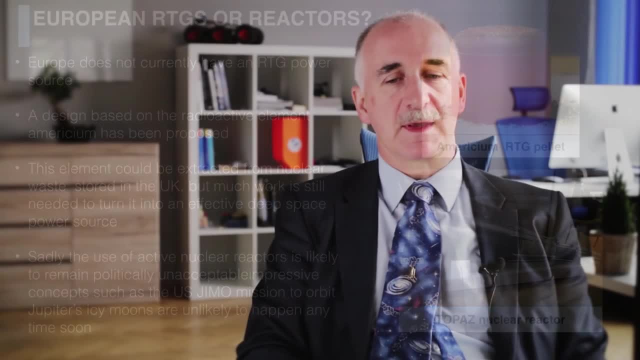 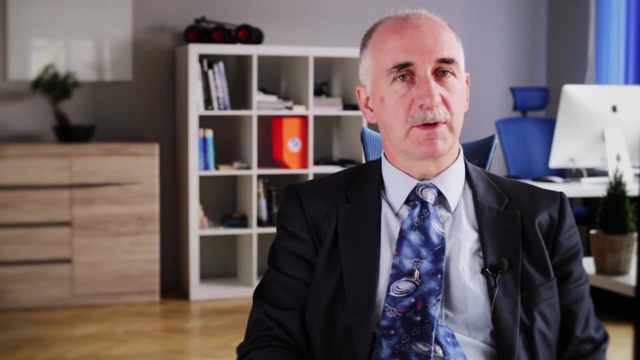 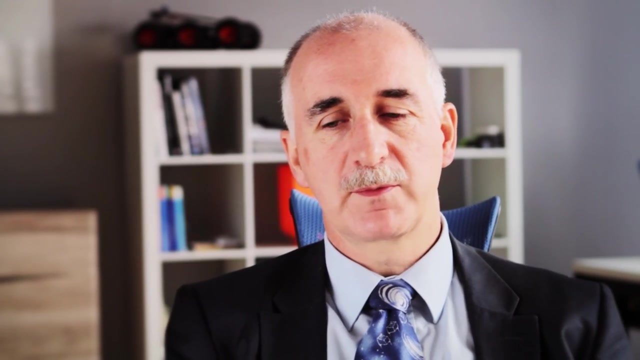 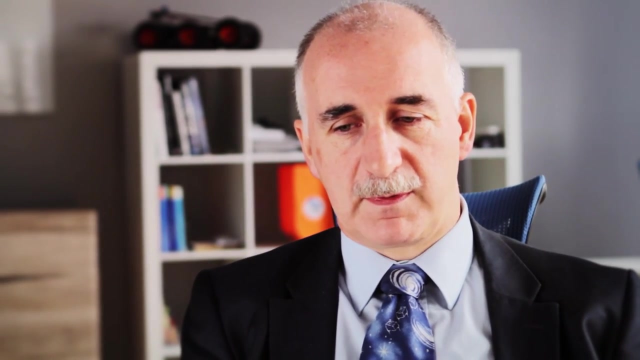 actually operate them in orbit. Where we don't think we're likely to go is the use of active nuclear reactors in space. The Russians tried this with a system of reactors called topaz, which were used to power some of their radar ocean reconnaissance satellites in the past. That sort of technology. potentially provides amazing amounts of power, but the difficulty is that you're now creating a radioactive hazard in low Earth orbit. The Russians recognised that and had an ejection system that was supposed to fire the reactor out of their spacecraft at the end of life. But unfortunately on one occasion The ejection system failed to operate. The satellite re-entered the Earth's atmosphere with its reactor intact. It landed in Canada and the Canadians took exception to the Russians dumping radioactive debris on their country, And at that point I think the Russians realised that it was politically unacceptable to do things like that. 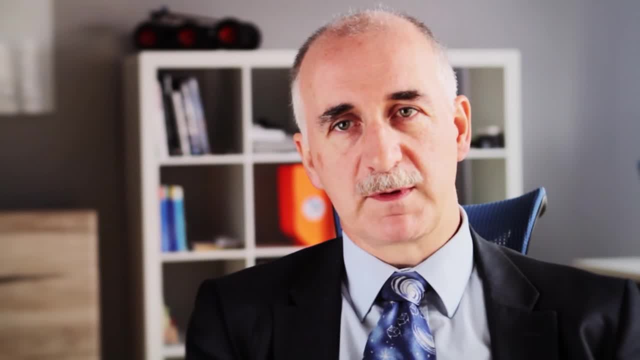 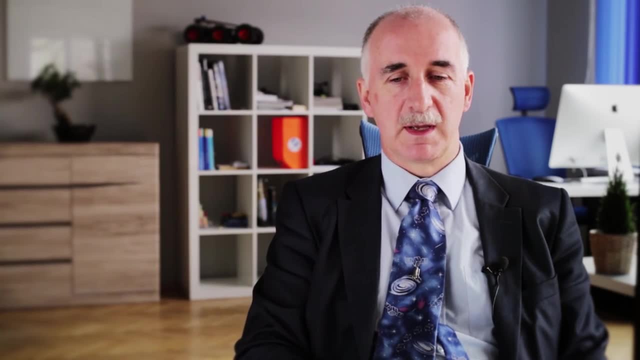 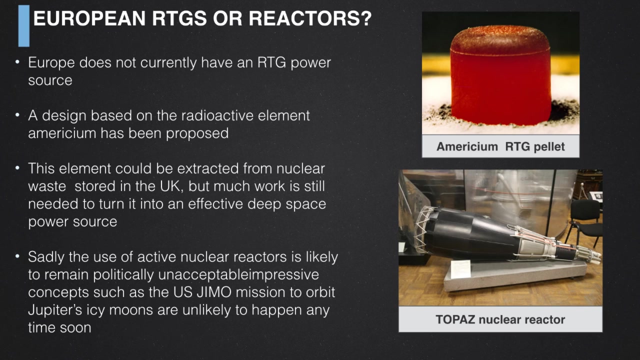 It is a bit of a shame, though, because some of the most interesting outer solar system concepts that have been proposed over the last few years, including a US mission that was also intended for Jupiter called GEMO, looked like an absolutely fantastic mission, And the reason it looked so impressive was because it had a nuclear reactor. 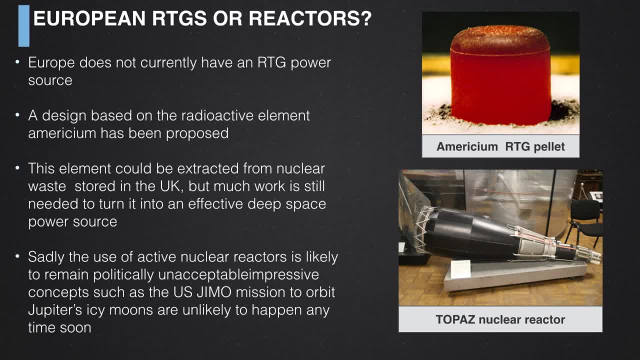 and was able to do an awful lot with the power that it would potentially have had available. But due to political pressure, it was decided that, even though the reactor wouldn't have been switched on until the mission was on its way away from the Earth, 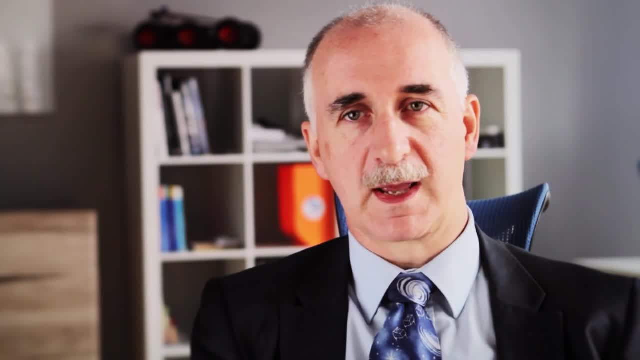 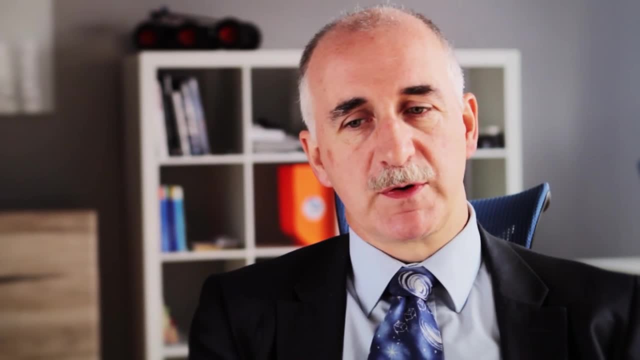 the political lobby was such that they couldn't get permission to actually build the spacecraft in the first place. Obviously, once you've got power, you need to store power. A lot of satellites in low Earth orbit pass in and out of the Earth's shadow. 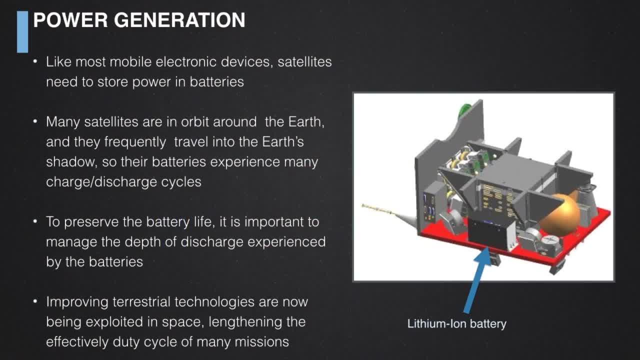 They go into eclipse and they're not generating power directly from their solar panels, So you need to have batteries. Again, the drive of terrestrial technology is improving things from our point of view, So we used to use NICAD batteries- rechargeable. 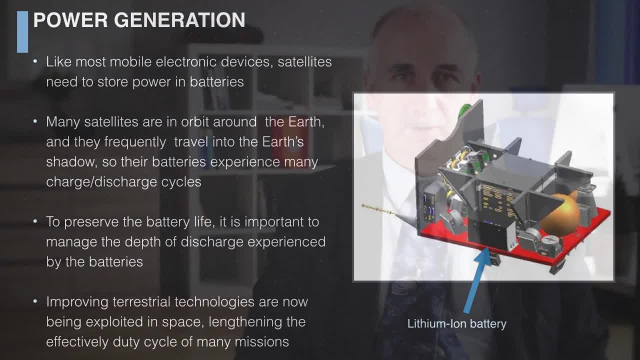 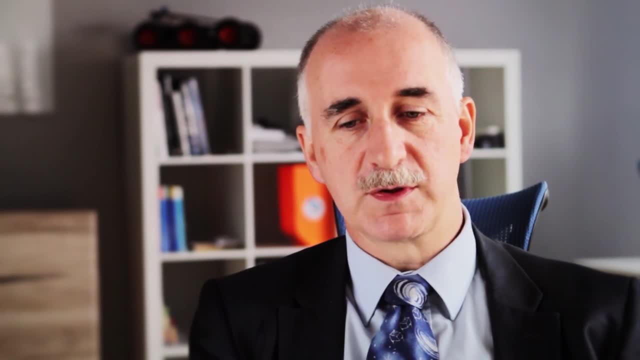 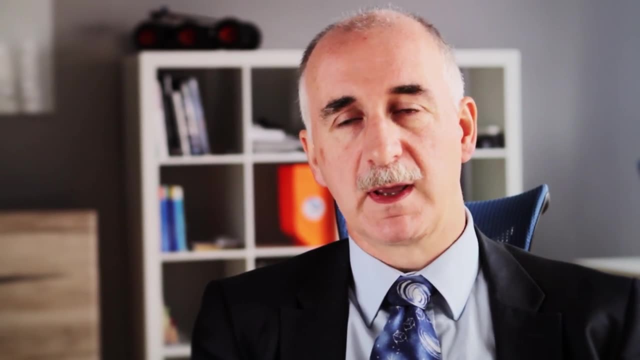 But now we've moved to using lithium ion batteries, which are the sort of battery technology that you find in quite a lot of mobile phones, And those batteries are more efficient, And so we have an improvement to the duty cycle of the missions that we're doing. 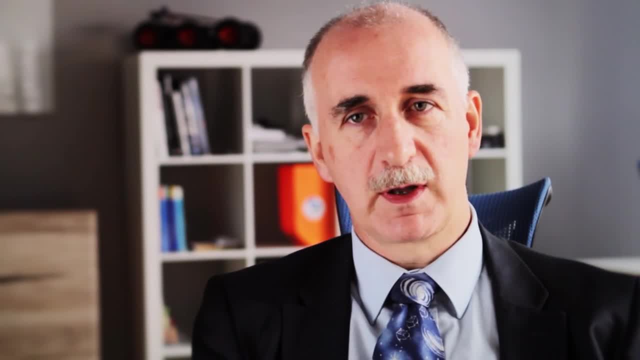 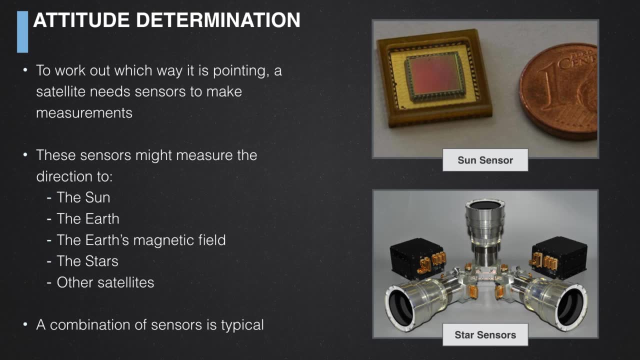 We can actually switch the satellite on and have it operating for a larger proportion of its orbit as a result of these improving technologies. The satellite then has to figure out which way it's pointing, So attitude determination is clearly important. Various reference sources can be used to determine which way you're pointing. Large and obvious things like the Sun, the Earth, can be used. The Earth's magnetic field using a magnetometer is another technique that's been widely exploited. The most accurate pointing comes from using stars with a star camera, which provides you the greatest angular determination capability. 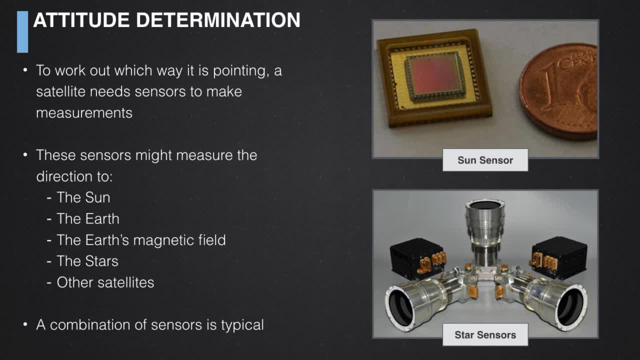 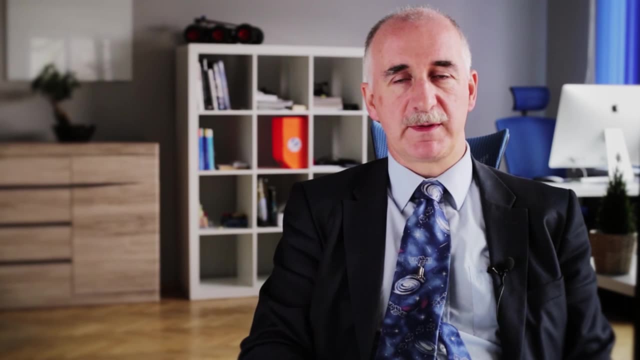 And it's even possible to use the transmissions of other satellites like GPS. If you measure the phase of the incoming signal with multiple GPS receivers, you can determine your attitude to some level of accuracy, Having worked out which way the satellite is currently pointing. 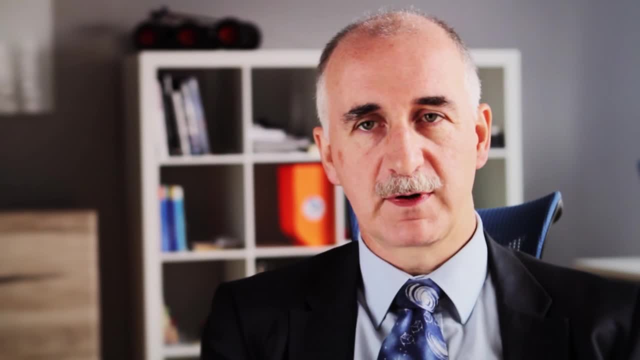 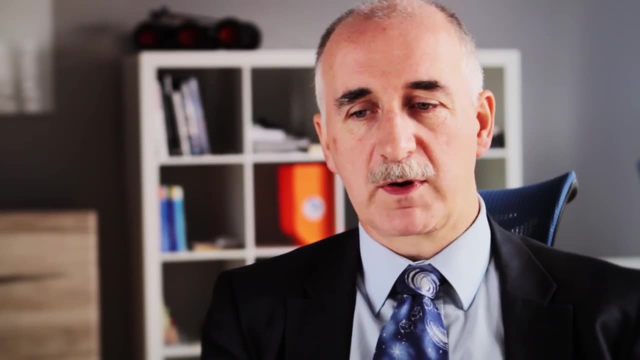 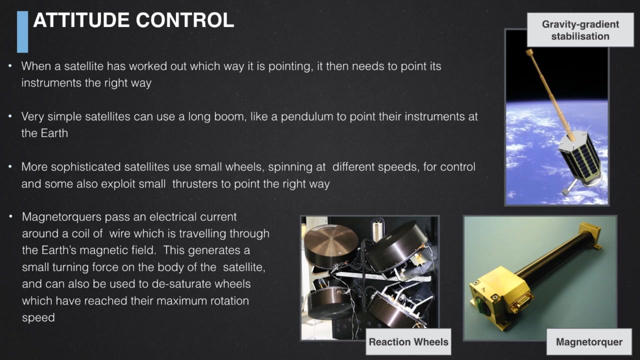 you may wish to orientate the satellite differently, And so you need an attitude control system to deliver that capability. Historically, some satellites have used very, very simple systems like a gravity gradient boom to achieve this. This is essentially a long deployable boom. 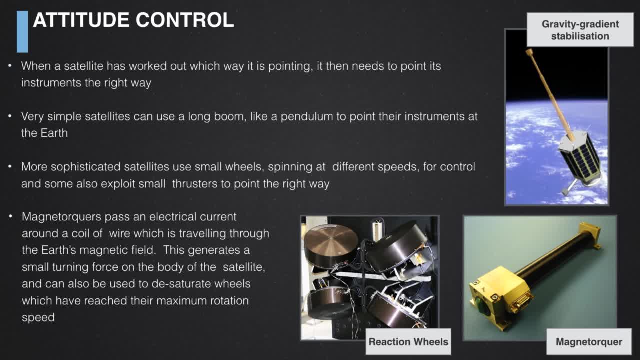 that acts a bit like a pendulum in low Earth orbit. The gravitational attraction on the body of the spacecraft at the bottom is very slightly greater than the gravitational attraction at the top of the boom And, as a result, a long structure like this is stable. 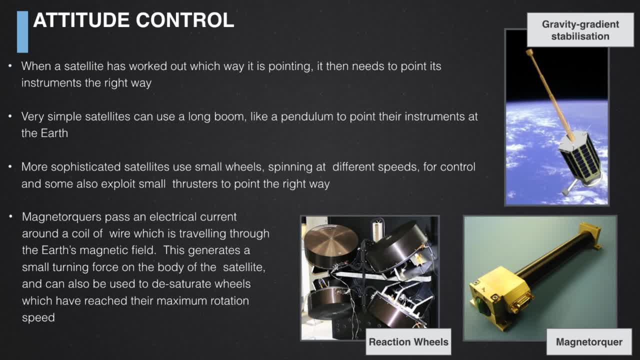 with the long axis pointing down at the Earth, which is useful if you want to keep the payload oriented towards the planet. But the Earth isn't a perfect circle Or a perfect sphere, And so the pendulum actually behaves a bit like a terrestrial pendulum. It oscillates, And if you don't control those oscillations you get a variation in the spacecraft's attitude by a few degrees, which is tolerable if you're using a radio frequency payload, but probably not sufficient for most imaging missions. So you need something to damp out. 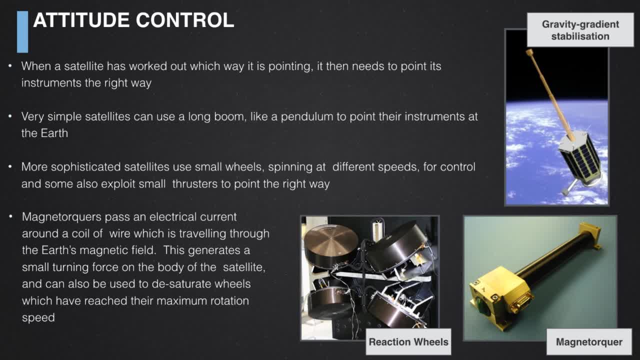 the oscillations of the boom, And typically spacecraft have used magnetometers to do this and magnetorquers. So you measure the Earth's magnetic field with a magnetometer and then you use a magnetorquer, which is essentially a coil of wire. 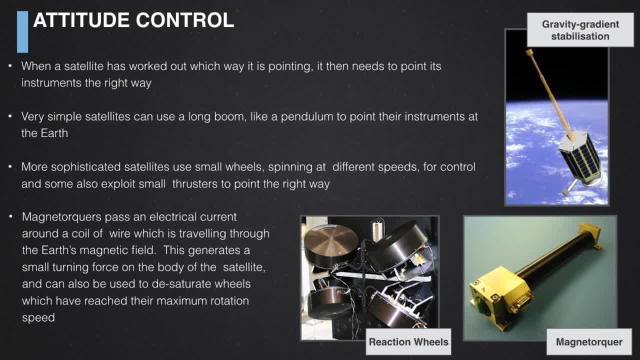 to affect the satellite's attitude. The way that you do that is, you pass a current through the coil of wire. It interacts with the Earth's magnetic field and provides a turning force which you can use to damp out the oscillations of the boom. 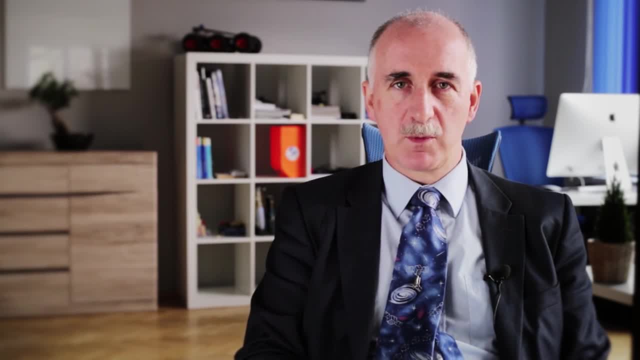 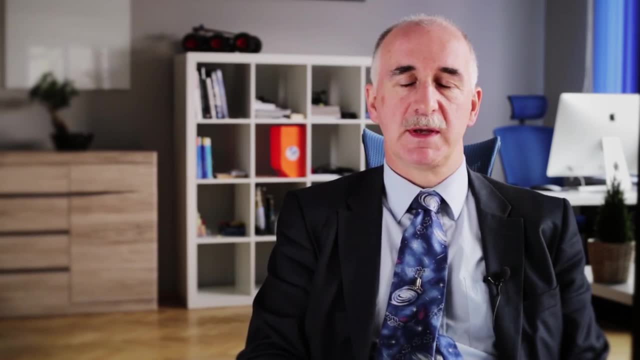 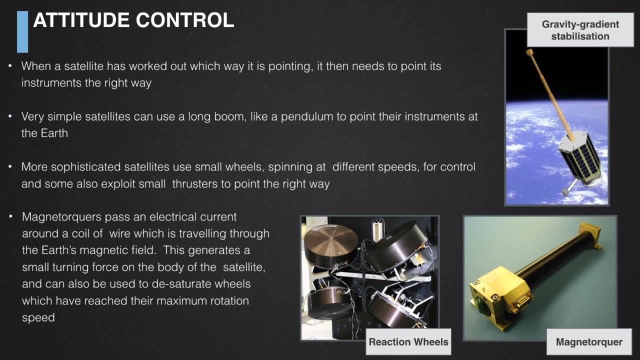 These systems, though, don't provide high precision pointing. If you want high precision pointing, you almost certainly have to go to some sort of wheel-based system, And the image in the bottom left of this slide shows a group of four wheels. Typically, you would have a wheel mounted. 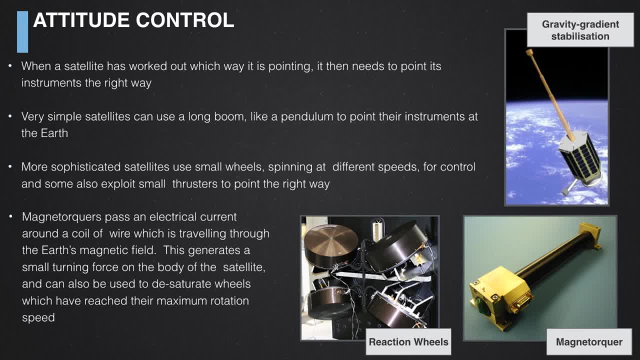 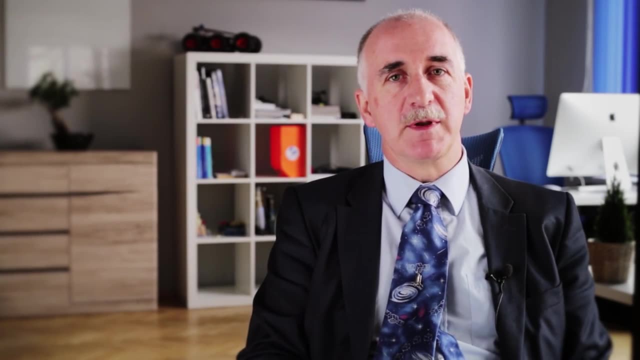 such that you could exercise control in each of the three axes of the spacecraft and then a fourth wheel mounted at an angle to give you some redundancy in the event that any of your three primary wheels were to fail. Temperature control is an important element of spacecraft design. 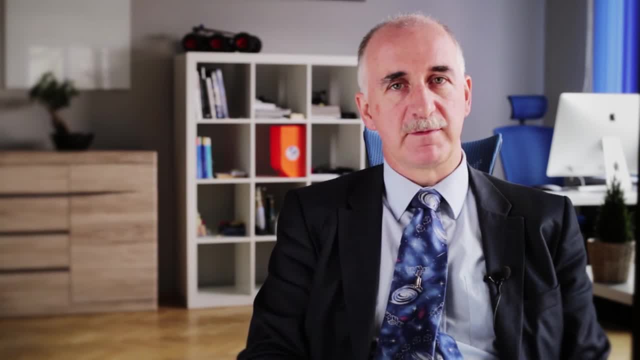 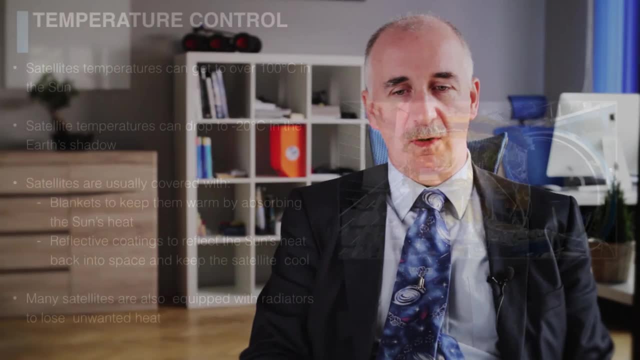 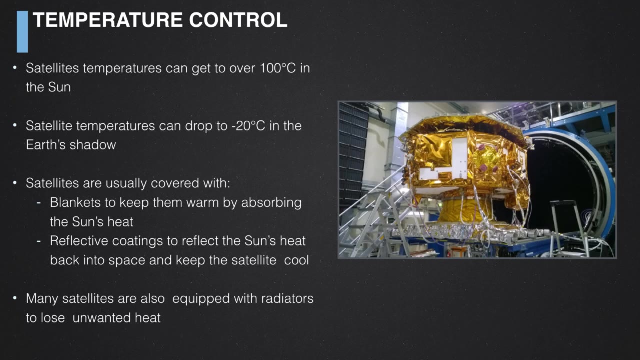 Many spacecraft are covered with reflective foils to avoid them getting too hot as a result of illumination by the sun. Clearly that applies when the satellite's in view of the sun. When a satellite in low Earth orbit goes into the Earth's shadow. 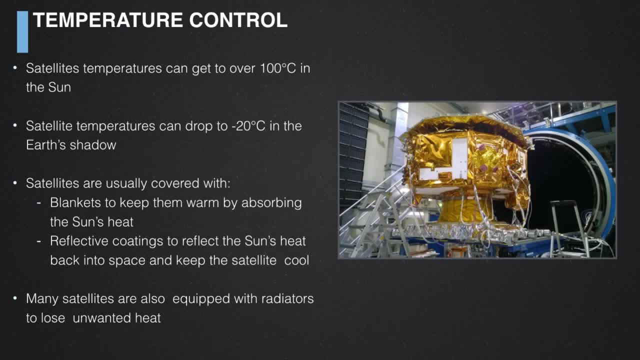 it starts to cool down. Satellites in low Earth orbit typically spend up to about 40 minutes in the Earth's shadow and can cool by quite significant amounts over that period of time. You can be at over 100 degrees when you're illuminated by the sun. By the time you come out of eclipse, your solar panels might not be as hot and might have dropped to a temperature of minus 20 degrees Celsius. That necessitates making sure that that thermal cycling on the solar panels doesn't get translated into thermal cycling of the spacecraft's internal electronics. 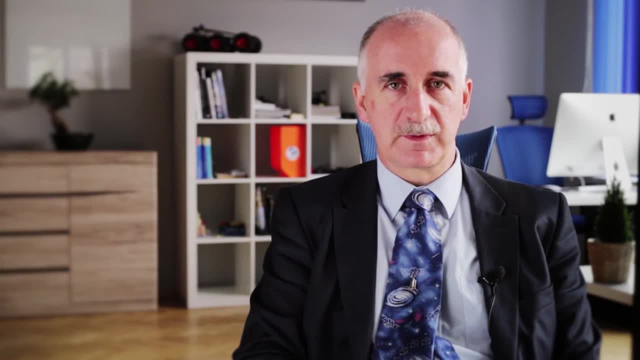 And, as a result, insulators are used to make sure that that doesn't happen, And the aim is to try and keep the internal electronics on the spacecraft within one or two degrees of room temperature, because that's typically the sort of range of temperature. 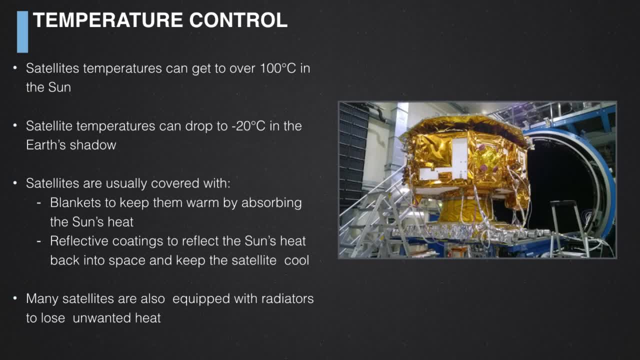 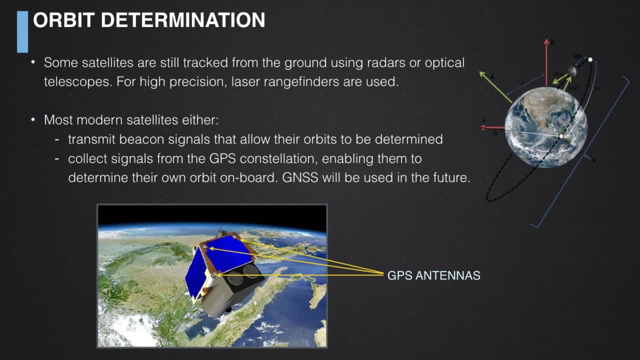 that the components are designed to operate in on the Earth. Orbit determination is the next challenge that you face. You need to know where your satellite is in orbit. In some cases, this is done externally to the spacecraft. Radars or telescopes on the ground are used to track the spacecraft. 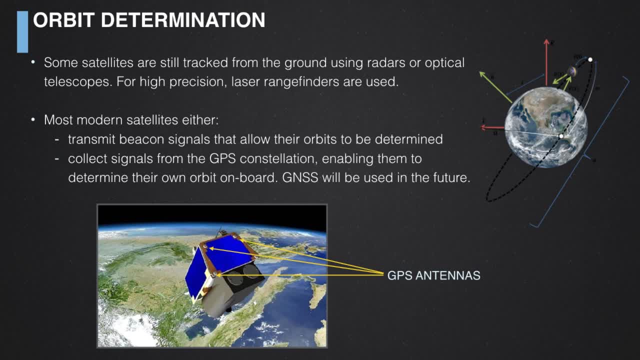 and determine where it is. But increasing numbers of modern satellites, especially ones in low Earth orbit, either transmit beacons that allow them to be ranged or use GPS receivers. So they act as subscribers- mobile subscribers- to the GPS signal and determine their own position to an accuracy. 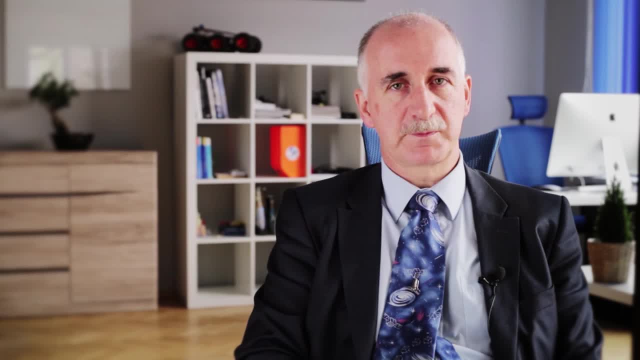 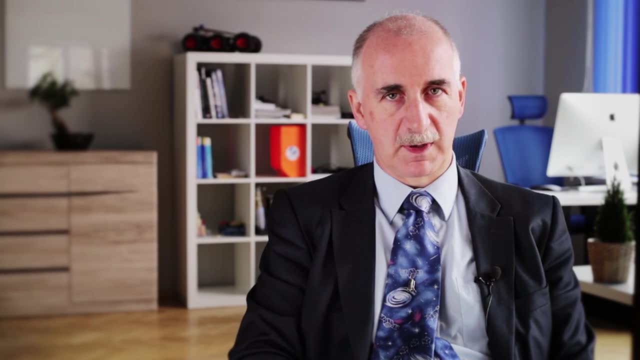 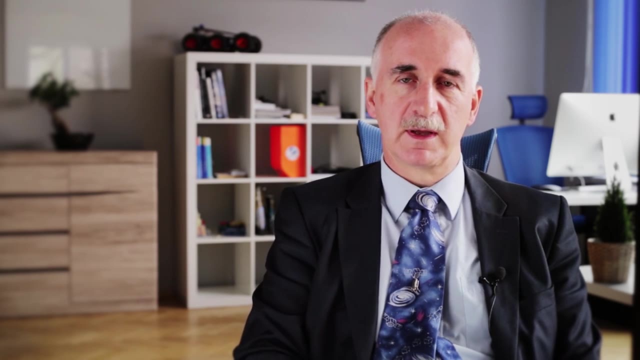 that's measured in single digits in meters, which is more precise than you can potentially track them from the ground using a radar. So the knowledge of the precision of spacecraft in low Earth orbit is improving as a result of using GPS And, in the future, the other navigation systems like Galileo. 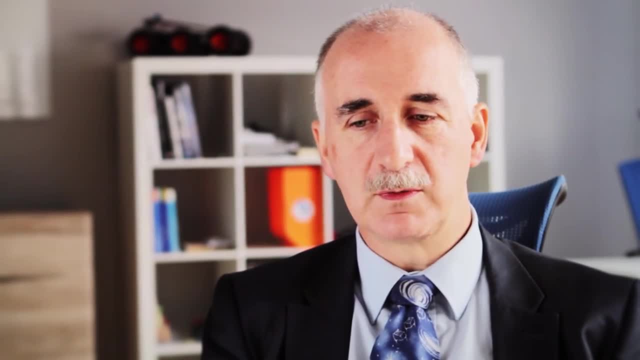 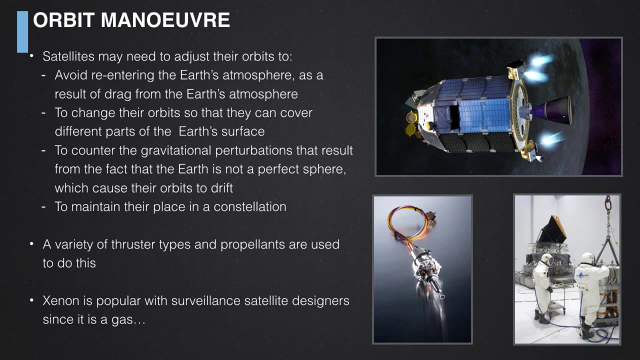 will also be exploited to provide precision orbit knowledge. If you've determined your orbit and you've decided that the orbit isn't quite the one you want, then potentially you need an orbit maneuver capability, And this can be provided by a number of different types. 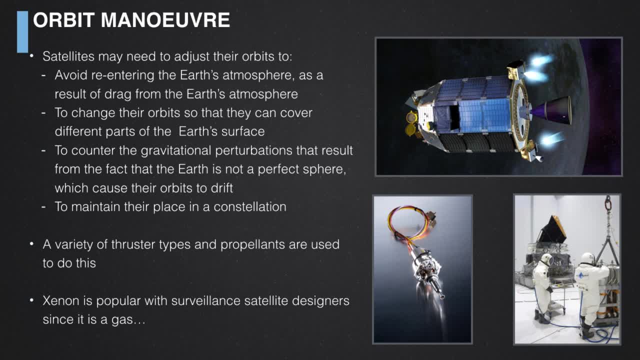 of propulsion system. Historically, spacecraft have used fairly toxic materials like hydrazine as a propulsion system, But in order to keep the costs down, it's better not to work with highly toxic propellants that lead you to a whole load of safety operations. 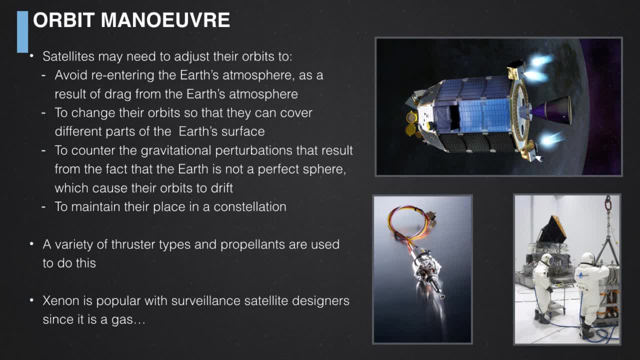 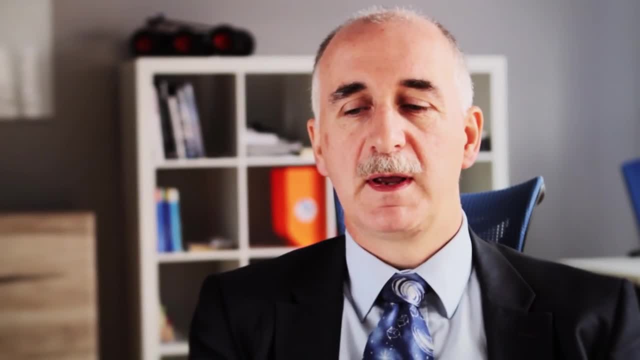 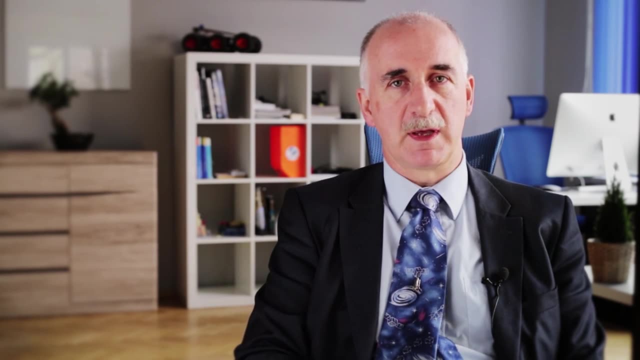 that you have to perform. So we've used inert gases like xenon, which is very safe and easy to work with. Essentially, our thrusters are known as resistor jets. You feed some of the propellant into a chamber where you heat it. 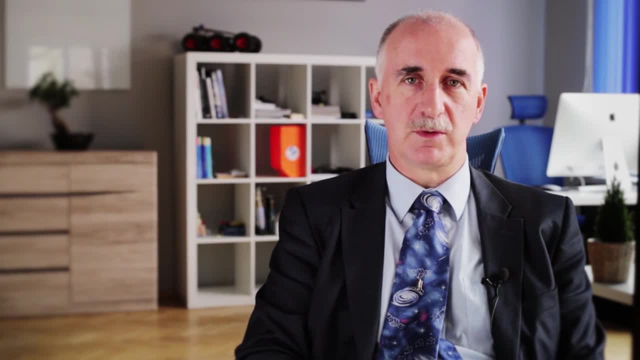 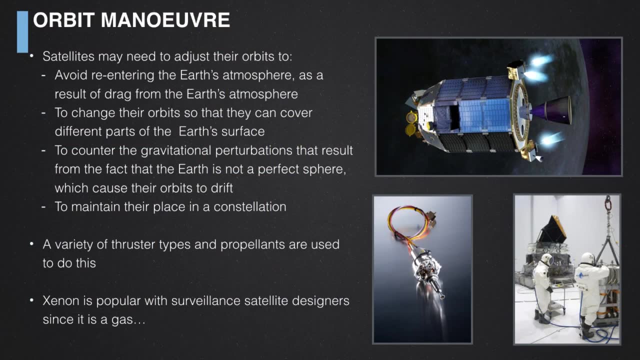 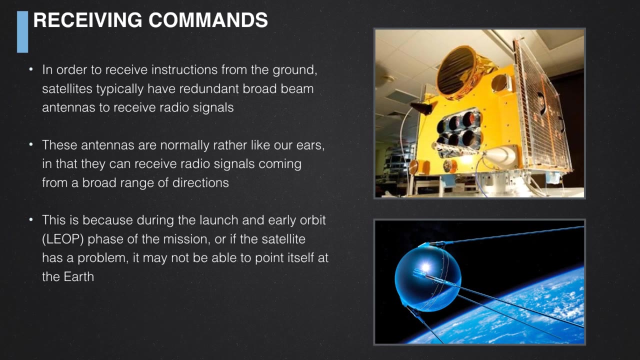 And it's essentially a kettle-like operation. You raise the temperature of the gas. That increases its pressure, so that when you release the gas the exhaust velocity is higher and you get a greater specific impulse from the propellant. You need to be able to tell your spacecraft what to do. 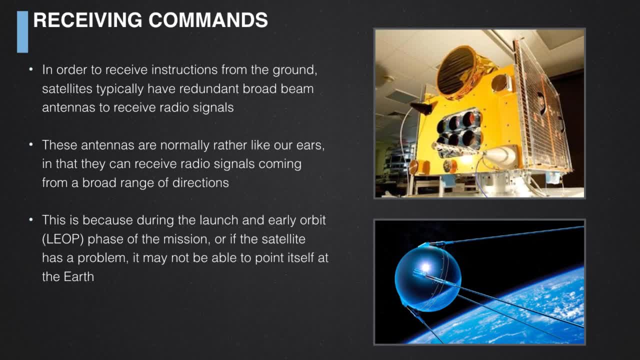 So you need to be able to send it commands And most spacecraft have redundant antennas on to receive commands, So rather like a human being with two ears, a spacecraft will typically have a pair of antennas on for receiving commands And in particular during the early phase of the mission. 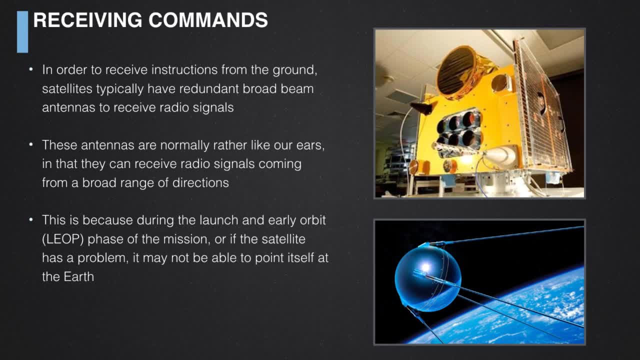 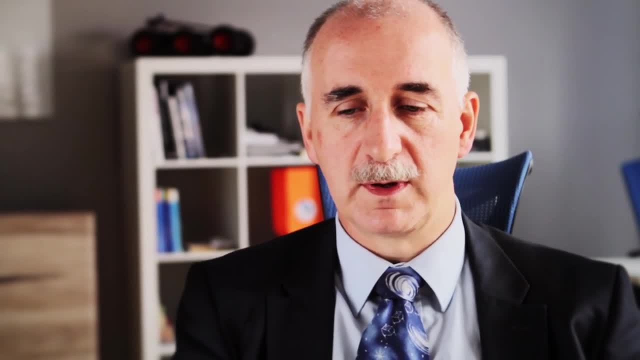 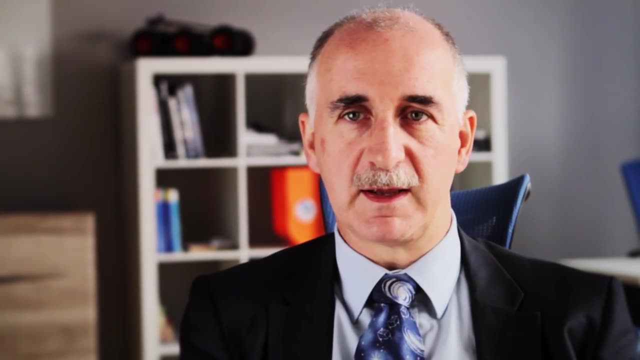 called the launch and early orbit phase. the spacecraft may not yet have stabilized itself, So you may have received antennas on multiple faces of the spacecraft so that it can't get into an attitude where it's unable to hear the commands that are being sent from the ground. 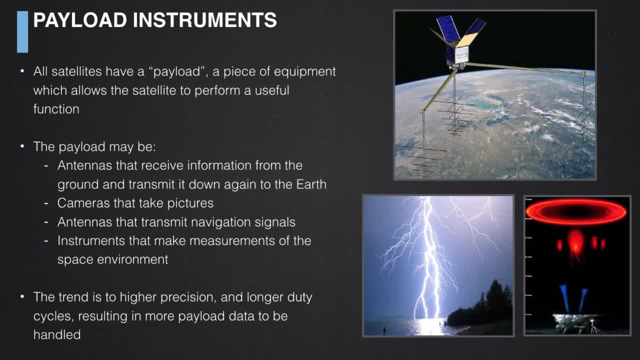 You put up a satellite for a reason. It has a payload that is collecting data of some form, And there are a variety of different types, some of which are listed on this slide. In general, a lot of spacecraft in low Earth orbit actually collect and store data. 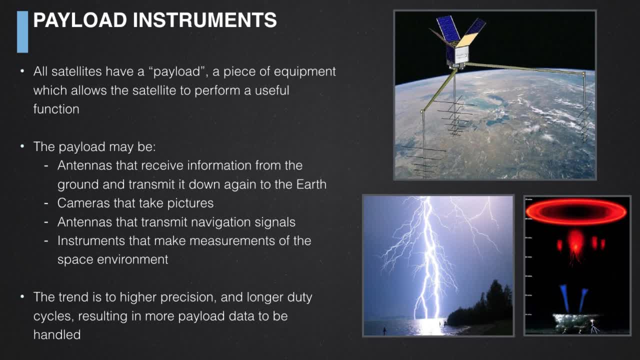 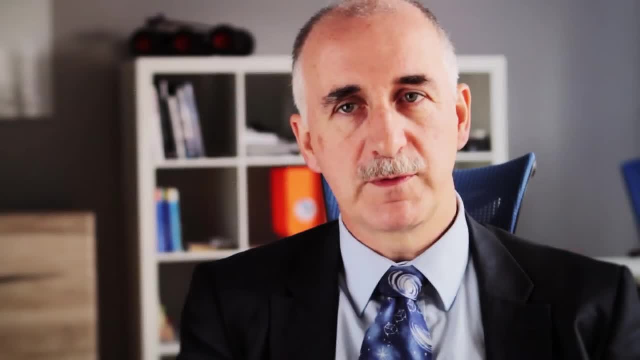 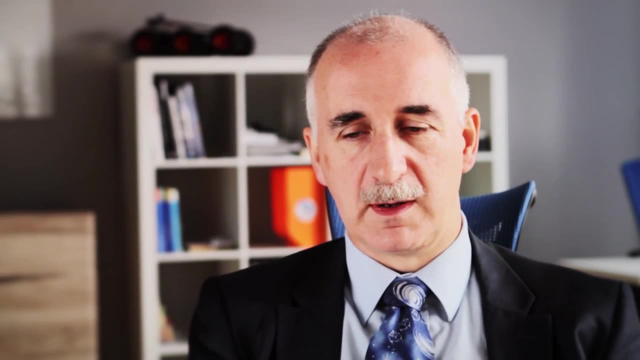 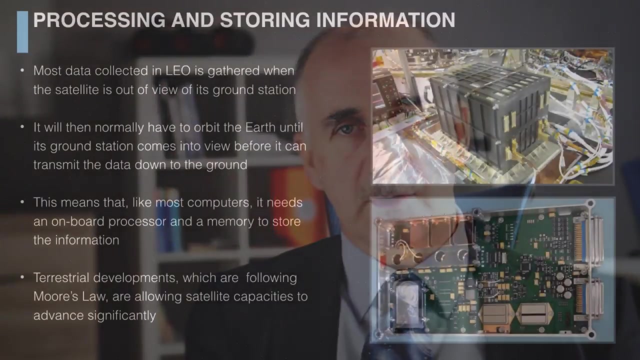 And the illustrations on this slide are a satellite that was used to investigate upward shooting forms of lightning that happen above thunderclouds. But clearly there are many different applications for remote sensing of the Earth from low Earth orbit. The trend is to increasing precision. 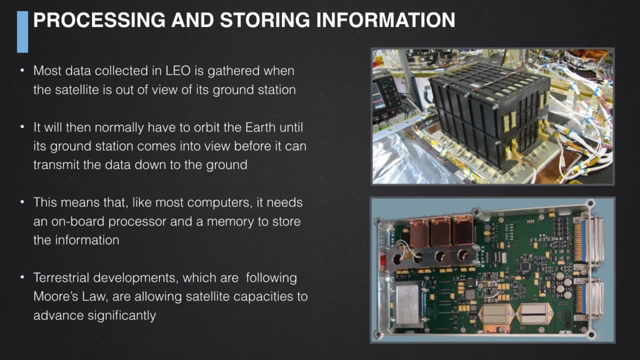 longer duty cycles. So that's progressively larger data files to be processed and stored, And that's what's covered on this slide. As time has gone by, we have been able to get progressively larger memory devices from the terrestrial microelectronics market. We're also able to fly progressively more capable. 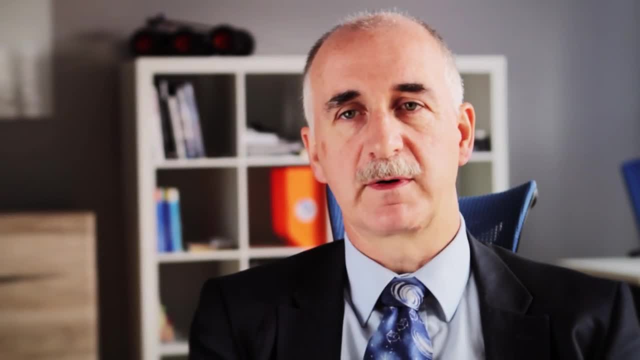 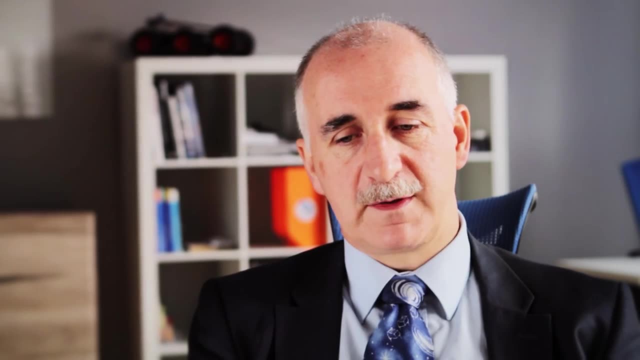 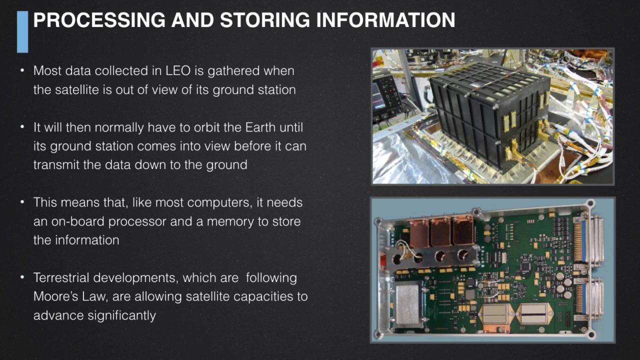 processors to handle that data on board the spacecraft and maybe even compress it before it's sent down to the ground. Our satellites are essentially following Moore's law, which is a law from the computer industry that says that processor power and memory size doubles every 18 months. 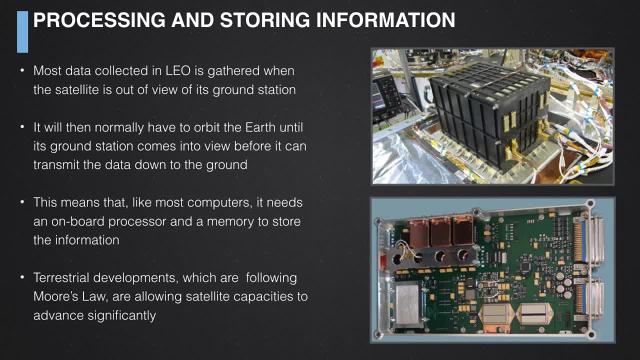 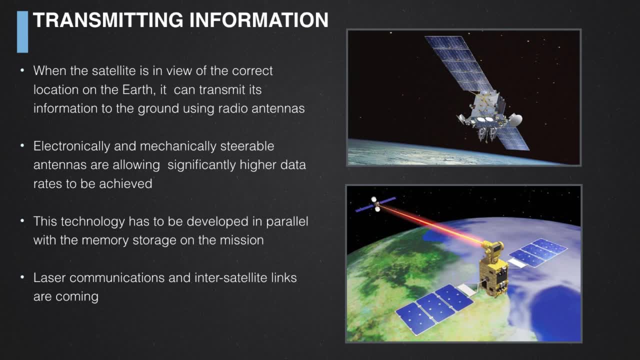 And our satellites show a similar pace of evolution. It's no use having all the useful information that the spacecraft has collected stuck on the satellite. You need to be able to get that data back down to the ground. So part of the design process for a spacecraft. 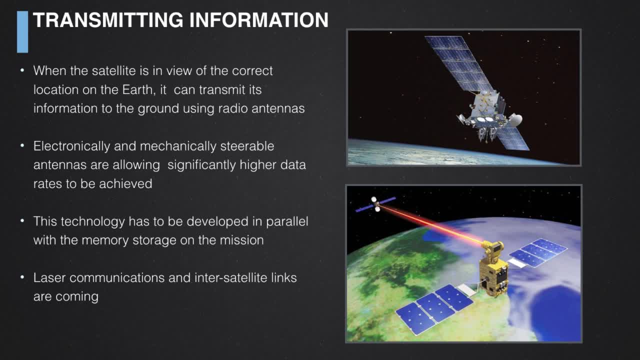 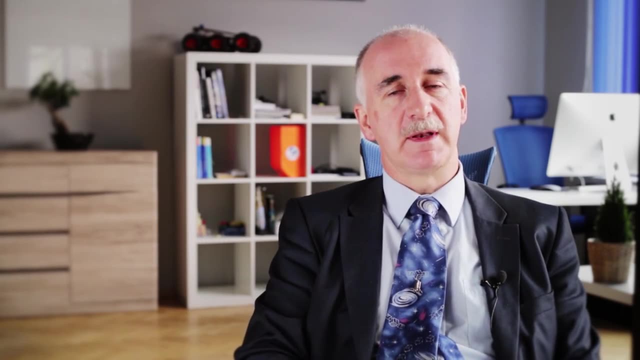 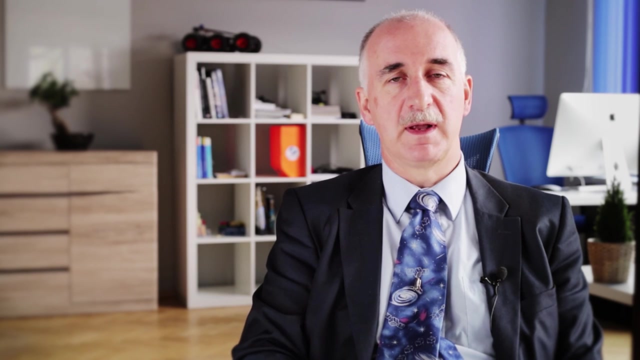 is to make sure that your data downlink capabilities are sufficient to unload the spacecraft memories as the spacecraft flies over its ground station. This is particularly important for satellites in low Earth orbit, which may pass over their ground station horizon to horizon in something less than 10 minutes. 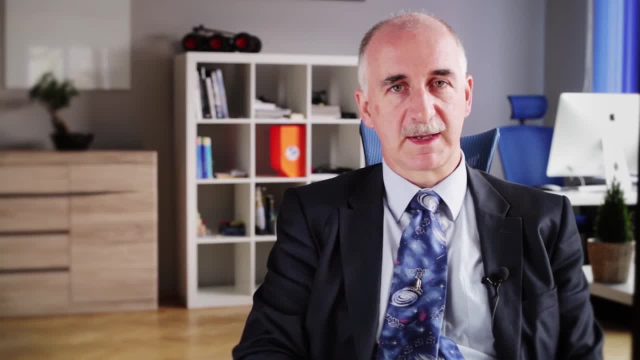 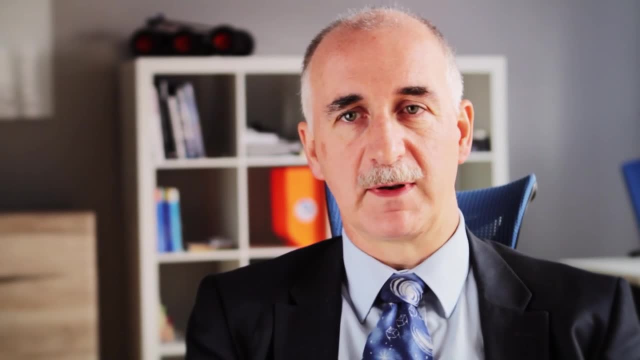 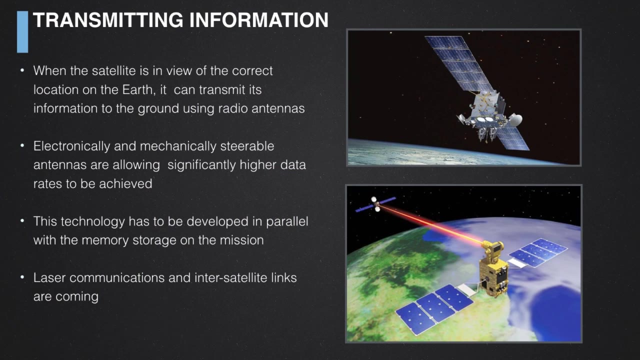 So you need to either use multiple passes to get the data down or make sure that your spacecraft has got a pretty high data rate downlink to empty the memory when the satellite flies over. But there are solutions to this particular limitation, and what I'll be talking about later is laser communications. 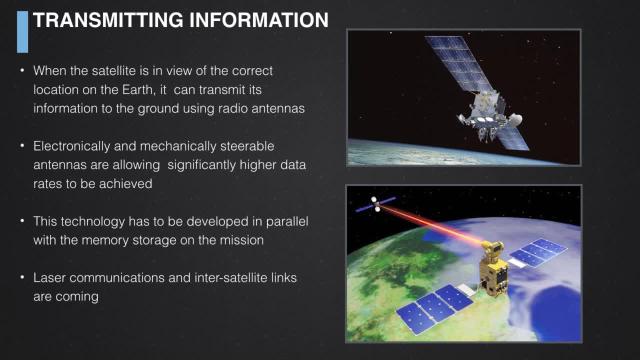 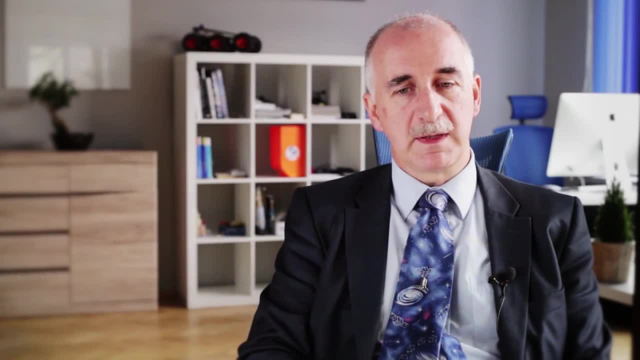 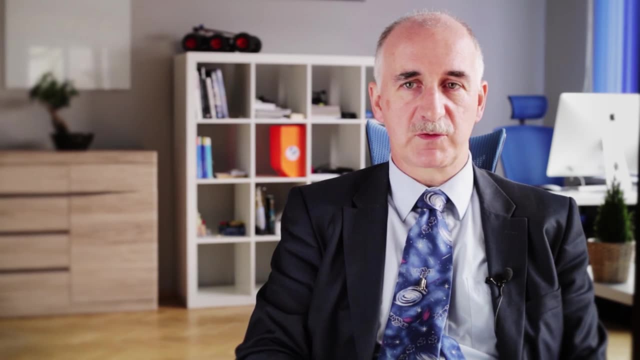 and inter-satellite links, which are two ways that satellites in the future will get over this particular limitation of the design. Finally, a spacecraft needs protection against the radiation environment that it'll see in orbit. Terrestrial microelectronics are not designed in general. 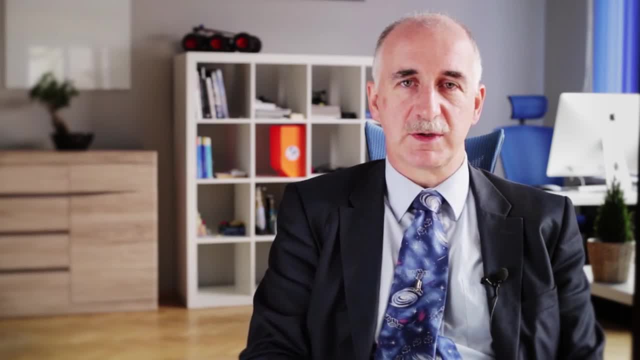 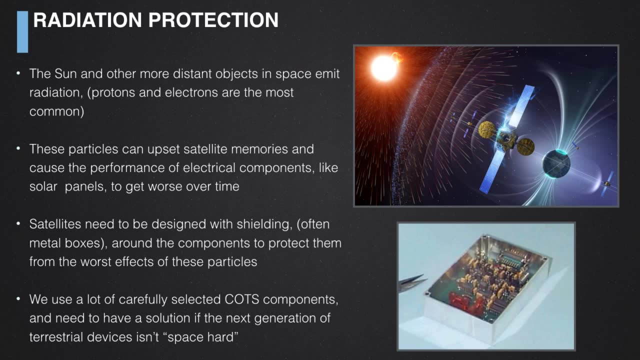 to accommodate a high radiation environment, And when we want to take terrestrial microelectronics into orbit and expose them to the particles trapped in the radiation belts and to cosmic rays, we need to think about how we handle that In the case of the relatively low energy particles. 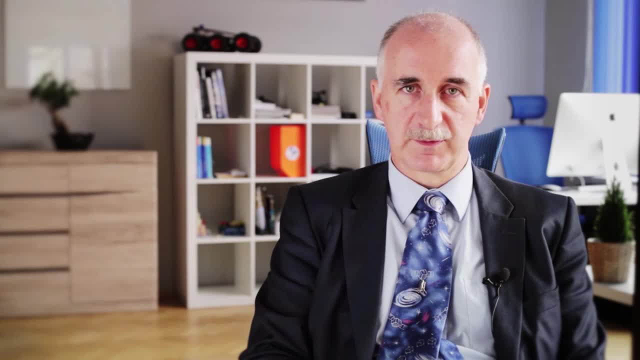 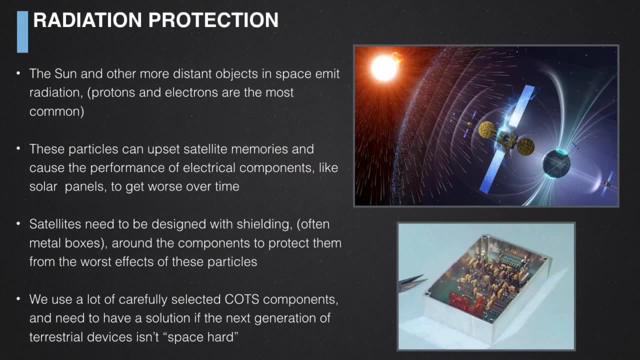 that come out of the Sun, the protons and electrons. we can generally shield those out using metal boxes around the components, which is what's illustrated here. The much higher energy cosmic rays that are generated well outside the Solar System are a different sort of problem. 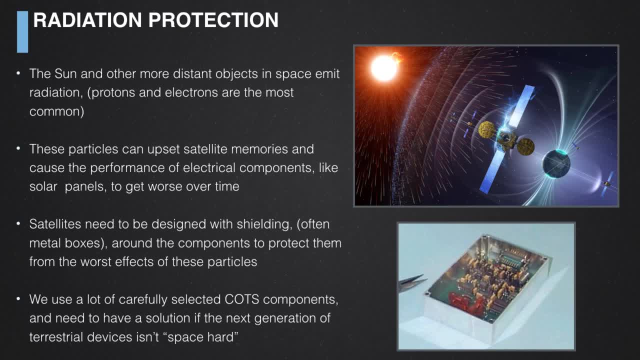 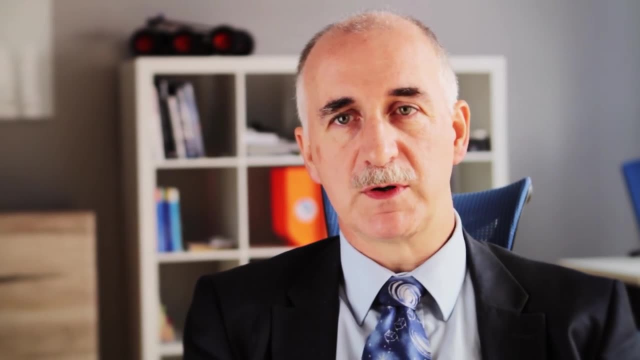 It's very hard to shield against those and as a result we tend to try and handle their effects in software. So an incoming cosmic ray might create what we refer to as a single event upset, a corruption of a memory state which moves the memory state from a one to zero. 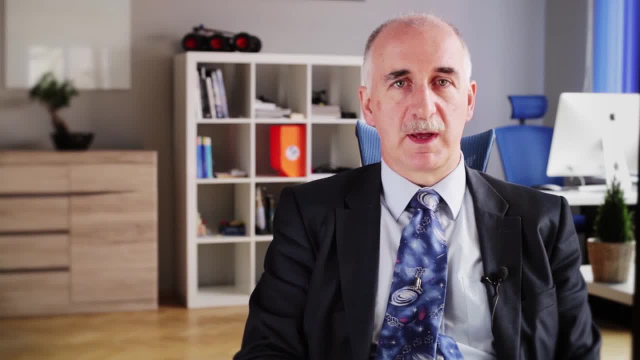 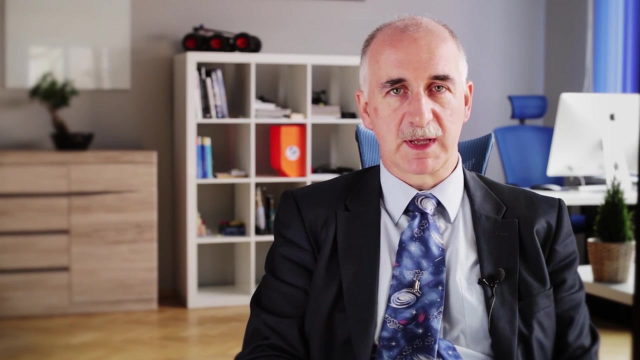 or vice versa, And we typically use majority voting on the spacecraft to resolve this. We would collect data, write it into three separate memory locations and then routinely compare the data in those three memory locations to make sure that it is still the same.